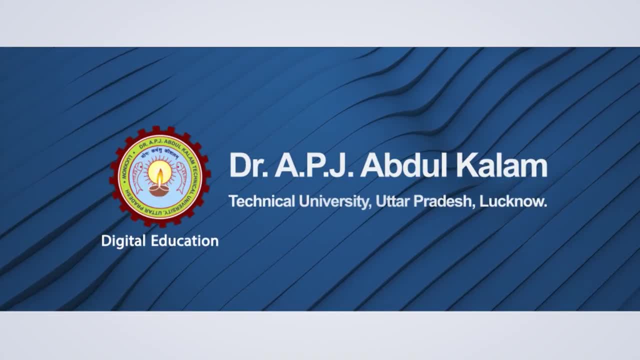 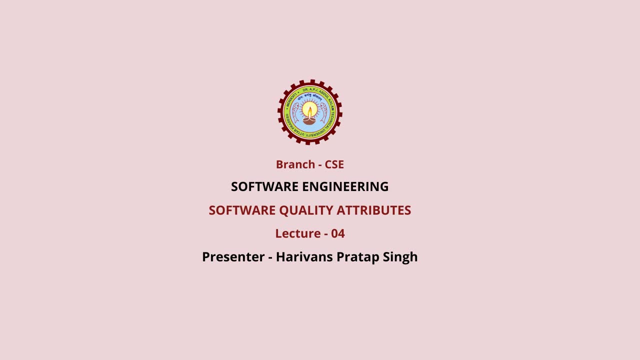 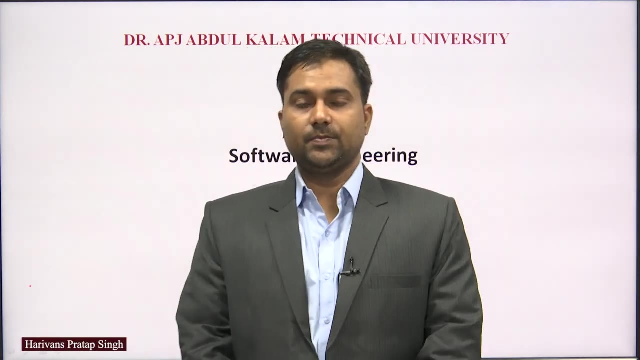 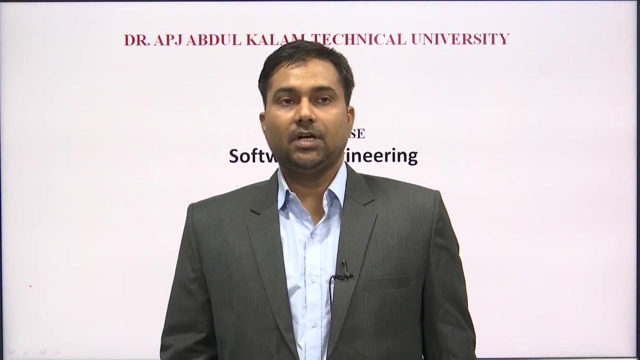 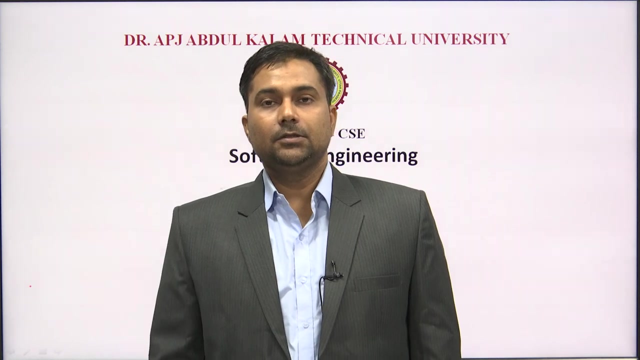 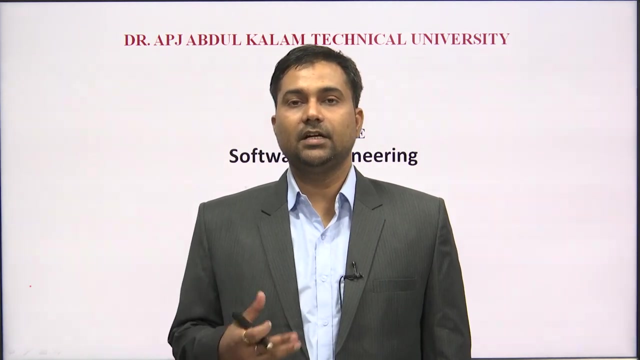 Hello friends, myself Hariwansh Pratap Singh. Currently I am working with ABS Engineering College, Ghaziabad. Today I have discussed software quality and its attributes. So, when we talk about software quality, what are the parameters based on which the quality of software 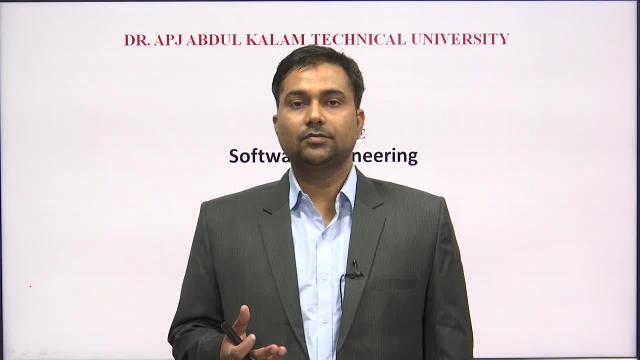 is decided right, And how do we measure software quality? If we talk about a good software, what are the parameters based on which the software is good or bad? right, So we are going to discuss in today's lecture. So what are the software quality parameters and attributes? 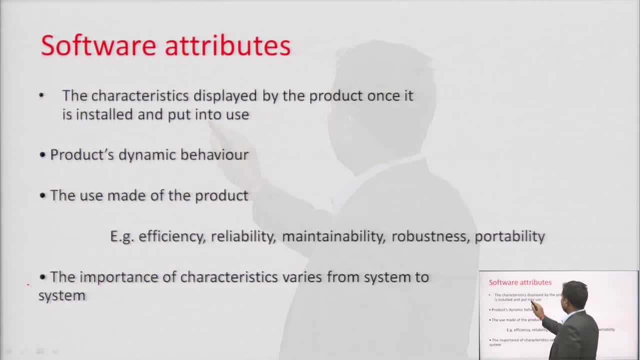 So, basically, what is software? quality attributes The characteristics displayed by the product once it installed and put into use. Whenever we install a software, it starts to be used. There are many qualities that are done, For example, when we use any website, it takes 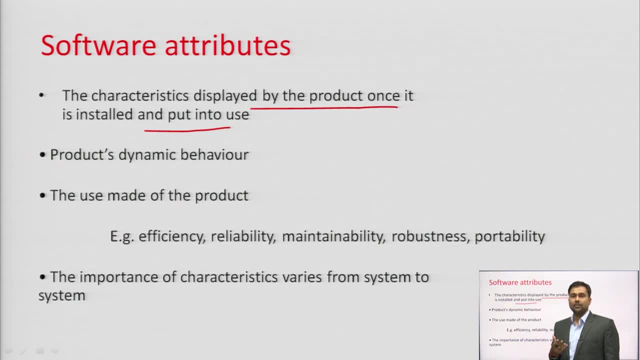 a long time to open it. its response time is slow, Right. Many times we wait by clicking it hangs. Sometimes the speed of the net is slow, but many times the speed of the net is correct. also, it is heavy because of the website, So this is a part of quality attributes. 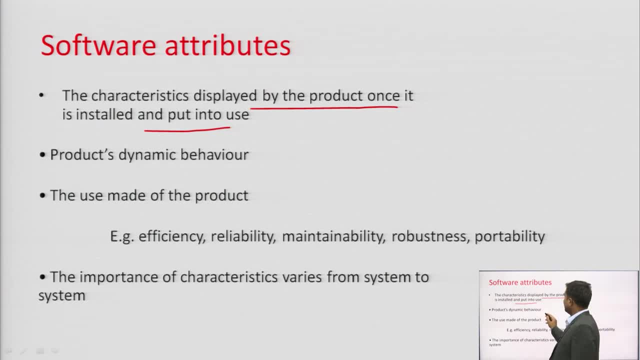 And product quality. Okay, Thank you very much. Product dynamic behavior. sometimes you have seen static website. dynamic website or any software is dynamically changing its response time. then dynamic behavior of any product is changing on run time. how is its performance coming right? it is running on multiple browsers. 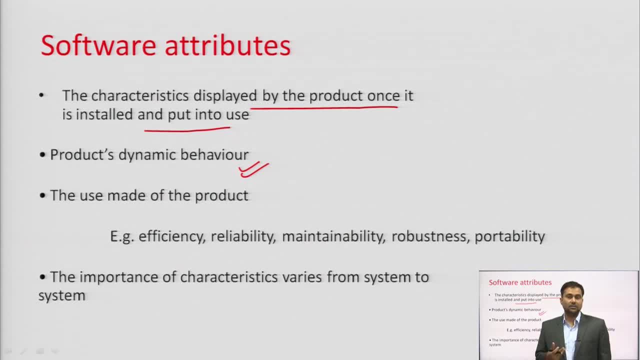 or not it is running on multiple operating systems or not, isn't it? the issue of compatibility is not coming anywhere. security is not bleached anywhere. if the security is bleached somewhere, then it needs to be fixed right. if there is a banking software, then why OTP has come? 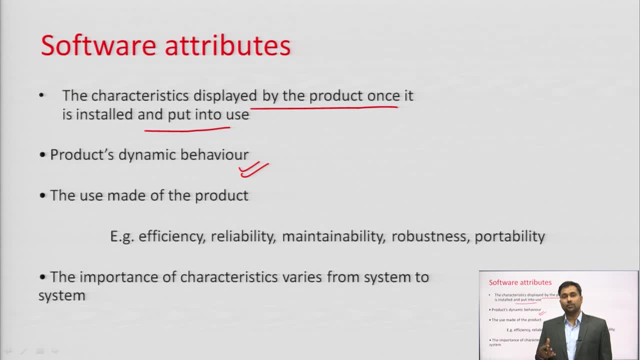 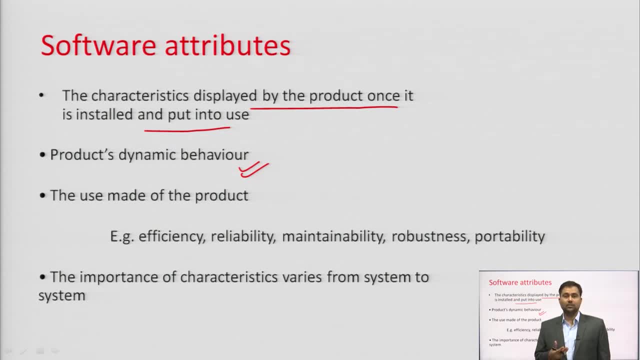 there and the reason is there, but it is not there. that may be in future, some maybe in future, some may have an opinion, maybe, etc. key: different, different reliability software, again, maintainability and robustness and portability. efficiency. maintainability, reliability, robustness and portability: yes, points of the software. 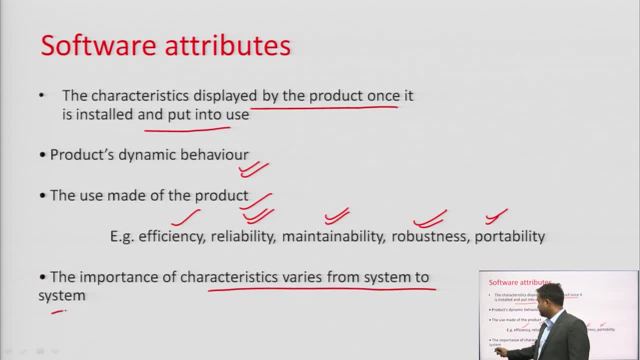 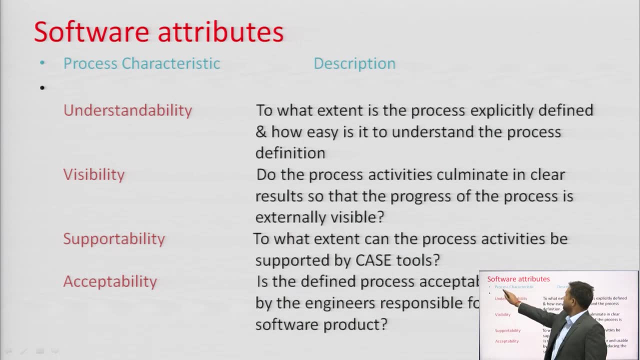 the importance of the characteristics, various form of the software system. basically software. first, understandability: to what extent is the process explicitly defined and how easy to use understand? and process definition of suppose that you have to send a message to someone through whatsapp or you have to type text. 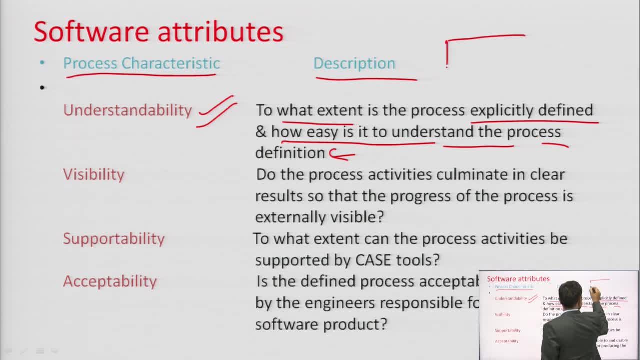 you must have seen an icon made in mobile, something like this. now, those who are not educated here also know the symbol by looking at it. GUI is made in such a way that it is a symbol to send a message. why? because earlier people used to send letters in envelopes. 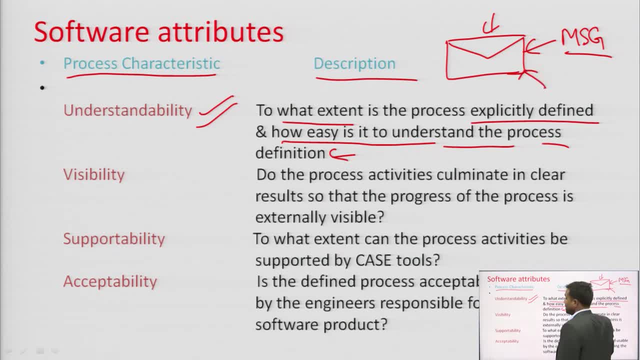 I used to send a message like this: so through this GUI, if there is an uneducated person, then he gets to know by looking at the symbol, how to use this mobile, how to send a message. right, so we develop understandability through our GUI. right, we make such a good GUI that it is understood by looking at the person in front of you. 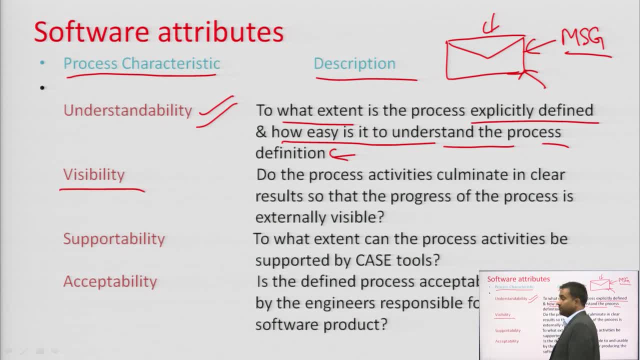 that this is its work: usability. now you must have seen many such software that you are searching for something but you are not getting it right. you must have seen many such websites where you are searching for some work in that website, so the visibility of everything should be proper. 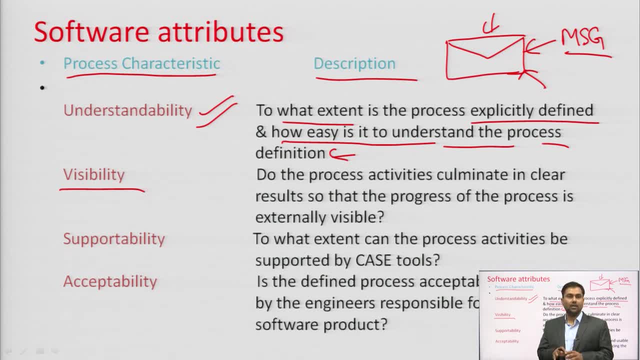 for example, if any user comes to your software, any stakeholder who is using this, any user, basically, if any user is coming to your software which you are developing, then it will be easily accessible, that thing which is required for it. so do the process activities. eliminate the clear results. 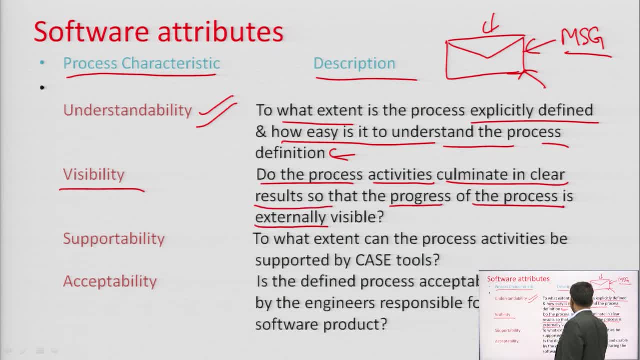 so that the progress of the process is externally visible. it will be visible from outside by inside, whatever you have to go inside. it is a step by step process but it will be easily visible, like if you do Facebook then you get to know the chat by clicking here. 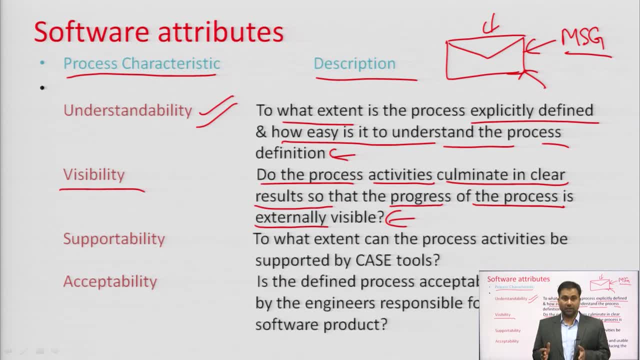 the chatting will start and when. personal chat. sorry, when you are doing personal chat, there is no connection with the other chat window of one chat window. whenever you are doing chat on Facebook, multiple chat window starts with multiple people. here the photo of the person with whom you are chatting. 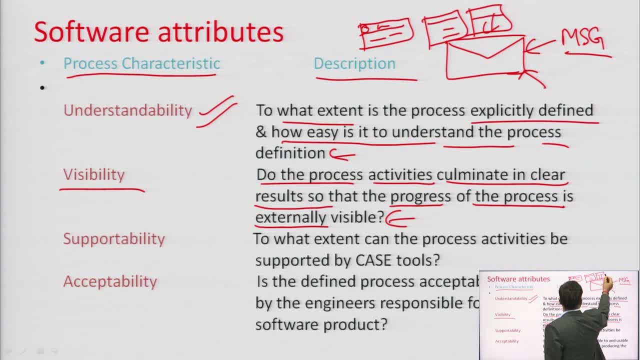 here the name comes. you are starting your own chat. I am talking about text chat, right? there is no connection between the two or the individual personal chat with individual person, right, but it is visible properly. you have logged in to Facebook and went to the home page then where to upload the photo. 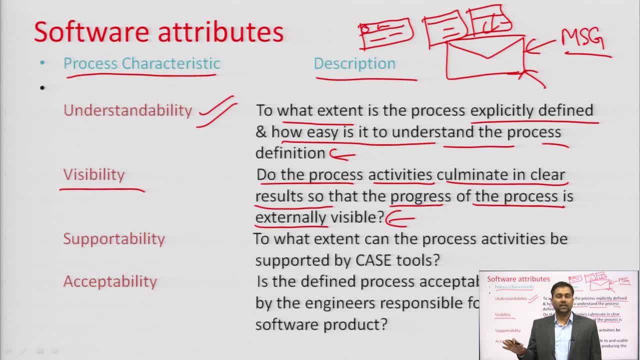 where to delete, where to update, right. where to post the wall like dislike, you have to do anything. there is also a search option, right, so the multiple modules are proper, visible. there are some websites of online shopping, right, so after logging in, when you go then what you have to search category wise. 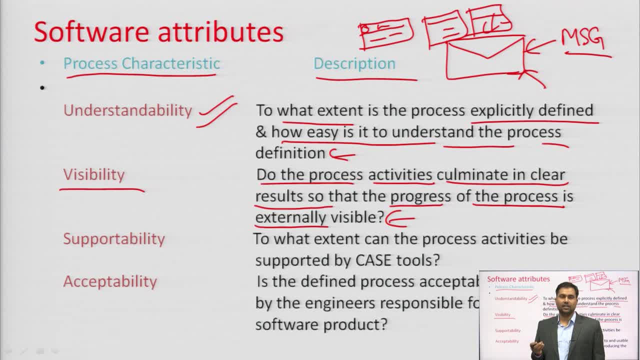 what shopping. you have to do. clothes, you have to do electronic parts. you have to do. vehicle, you have to do something. books, you have to buy whatever. so by going to the proper category you can search from the name of the writer of the particular book. price offers: 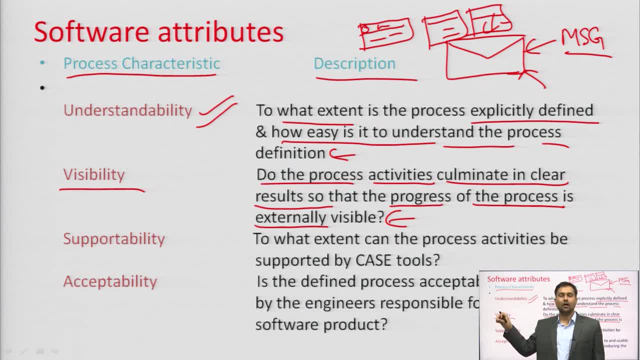 after that, adding the card each and everything is well organized and well sequenced. first you will log in, then you will do shopping, then you will add in the card, then the bill will be generated, then you will check your bill, then you will do payment, then the order will be placed. 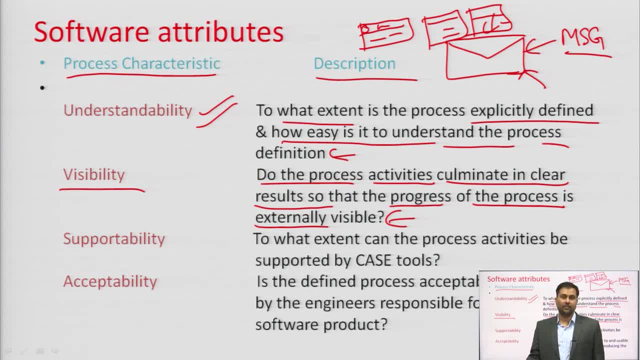 then you will do tracking of the order, then the delivery will be done. the message of successful delivery will come. each and every step is well organized and well planned. this what I have described to you verbally. you can take any online website, whether you take Amazon or Flipkart. 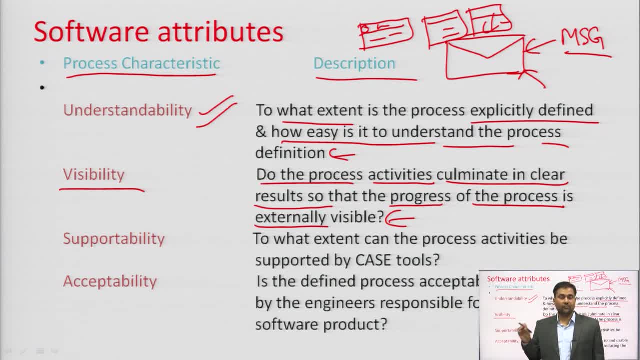 so like this, each and every software is well organized if we plan it properly, by planning proper architecture, by planning proper human, whoever is going to use the user, by understanding his mind set, we will plan so obviously it will be usable for him, it will be easy to access. 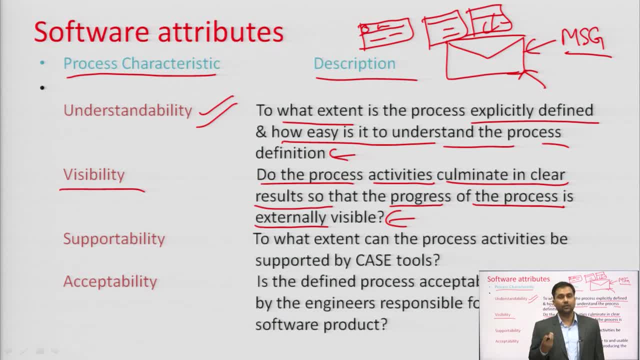 and visibility will also be proper. it is not available to search, so it will be quit on the website. multiple websites are not working because it does not have proper visibility. that is also quality parameter right supportability: to what extent can be process activity be supported by the case tools? 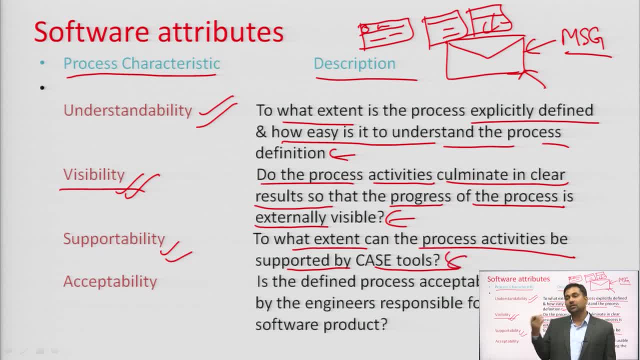 what are case tools? which converts design documents into code? IBM has made many case tools, IBM products, right, so there are multiple case tools which help in proper development process. they support your development process, like in tracing the whole project at what level the production is going on. development is going on. 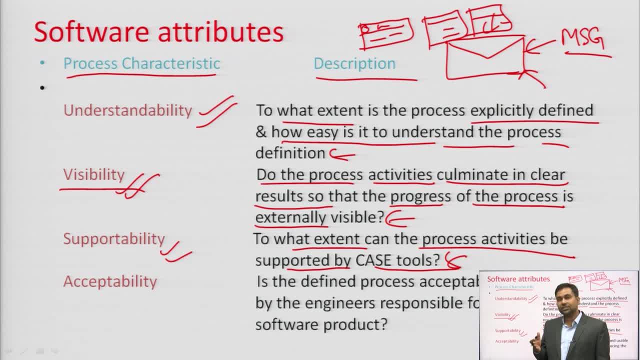 not production, actually development. so the development of software. how much we have reached in step by step process, whether it is going on in timely manner or not. for that also, case tools are made to make design document, to make UML document, to convert it into code. there are multiple case tools. 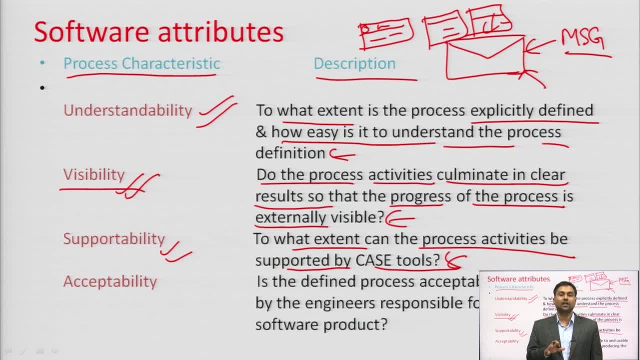 which support to improve the quality of software and in development, to save time and cost. they help in your development. in short, accessibility, acceptability. now what you have to accept, what to reject. this is also a challenge. is the defined process acceptable to and usable by the engineers? 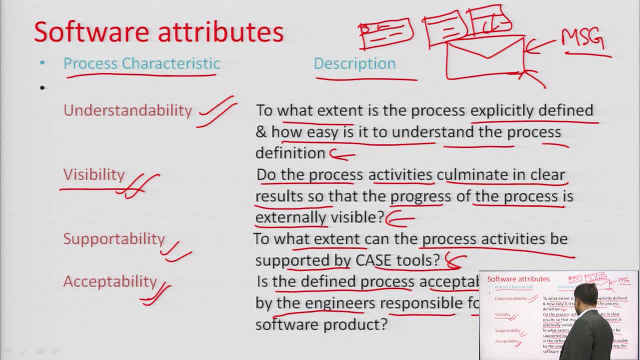 and responsible for the producing the software product means what? whatever software product you are going to develop in that engineering methodology, whatever process we are going to adopt, which software development life cycle we are going to adopt- according to the project to project it will vary, obviously, but that defined process, 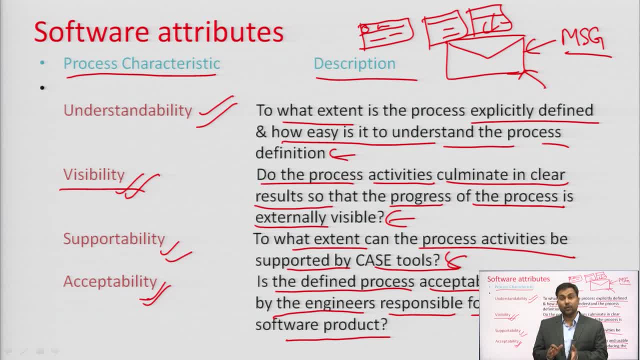 we have to accept it. whether it is going on in the process or not, whether the process is being properly followed or not means, after making the requirement document, have we gone to designing, or have we started designing first? if we are designing, then have we started coding also? 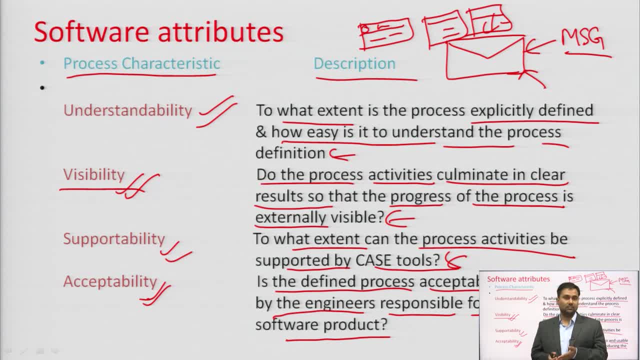 so the bugs which will come later- we have to change it completely- may be. we have to change it in the design, so change the code again. so our cost will increase, delivery time will increase, right? so we have to keep this focus. that what we are going to accept. 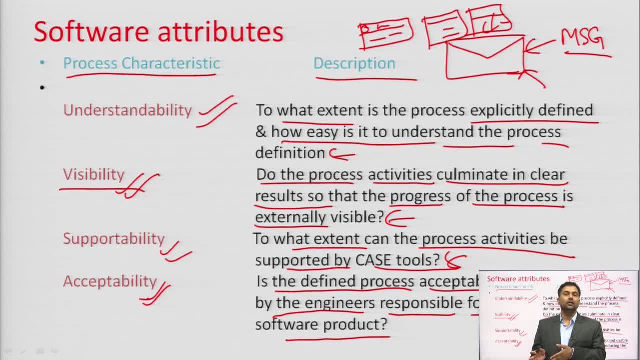 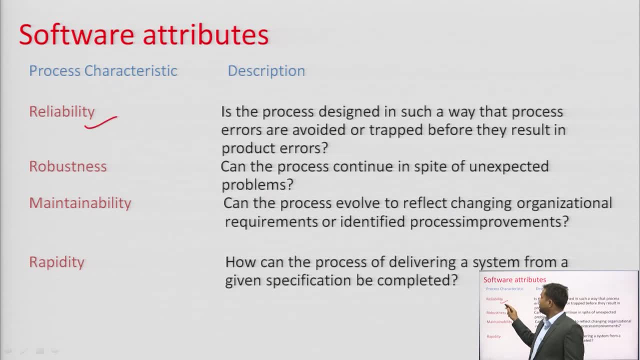 and the process which we are accepting. we have to follow it right again. few characteristics are reliability: is the process designed in a such a way that process errors and avoided or trapped before the result in produced error means if the software we are developing, the project, software, project product we are developing. 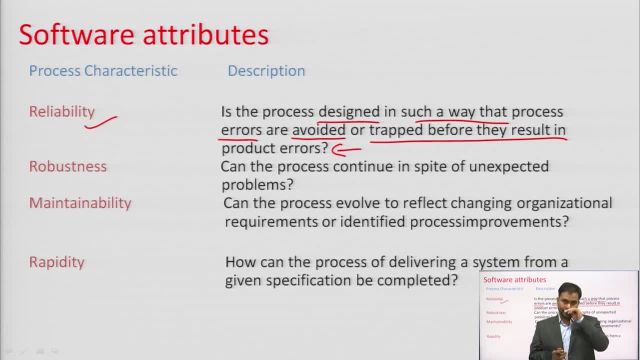 if, if we have done the proper testing in multiple ways, in multiple types of testing and fixed all the bugs, so before delivery we have fixed maximum bugs, maximum modules, whole software in running condition and trying to less bugs, less defects, then we deliver. so from this how much we will test? 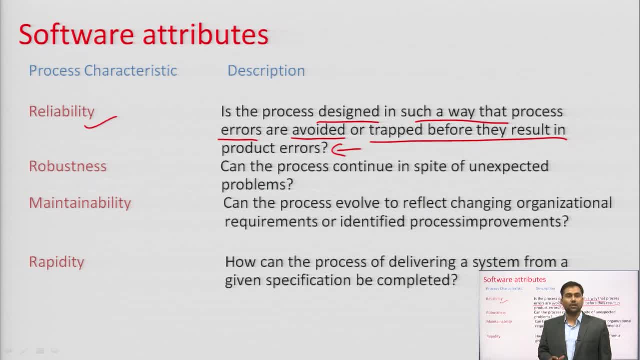 how many types of bugs we will test. how many testing we will do the relevant engineers test them. now what I will explain. first of all, after rendering that, our design will be good. we have gathered the proper requirements, we have refined it in multiple ways. after that, what we will do: 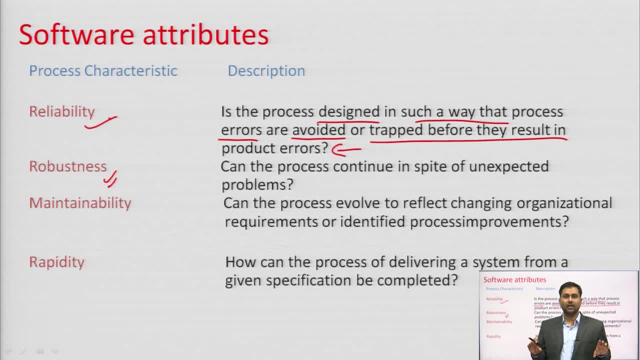 design. we will make proper design document. we will remove the shortcomings in designing. we will verify the design document properly. after that we will run the code and validate it. we will follow all the coding standards. after that, in our testing time we will remove the bugs on developer side and tester side. 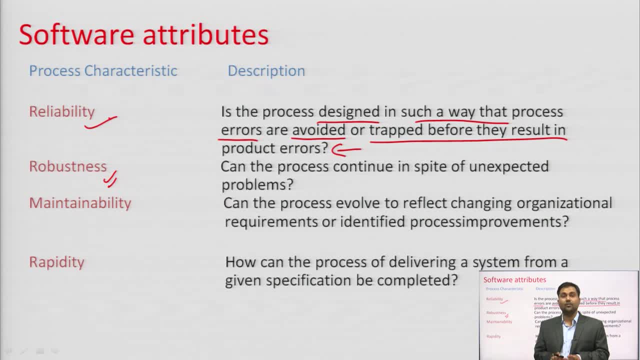 before delivering to the user, we will perform all the testing. we will perform all the performance testing. after that, the software product will be reliable and robust and we will update it in time to time so it will exist in the market for long duration maintainability. now this maintainability is little complex. 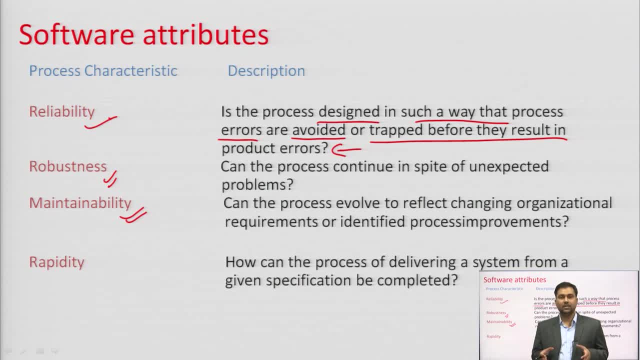 because this depends on the modularity absolutely. if we have developed the project through the modular approach, then if the modules are independent, like the difference of chat module, there is no difference of login. if you come to facebook after login on the home page, then there is no connectivity of login page. 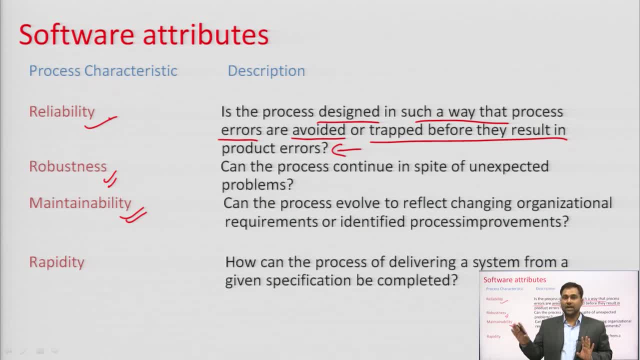 you just have to login. after that, the work of login page is over with the help of chatting. you just click on your online friends and type chatting. chatting starts. there is no connection with photo module. only photo will come and name will come from profile. that is it. 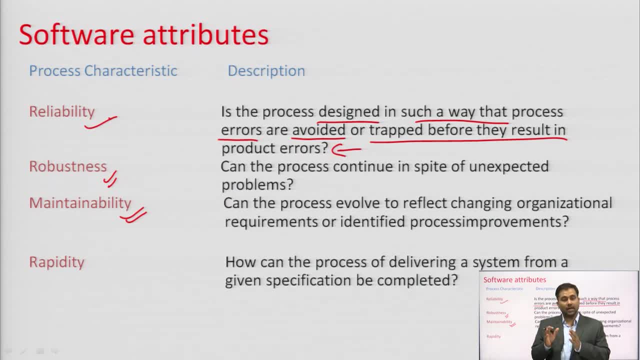 that is the integration of both modules. but if errors will come in the chat, then it will not reach in the login page because there is no connection between login page and chat, right? so that is the modular approach. so each and every module. if there is a bug in any module, 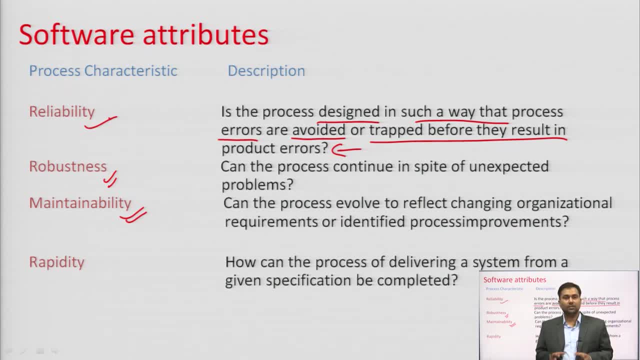 then it will not reach in the other one. that is the beauty of modularity. so if we have applied the modular approach to the design, then what will happen? the maintainability will be easy. if maintainability will be easy, then the testability will also be easy. 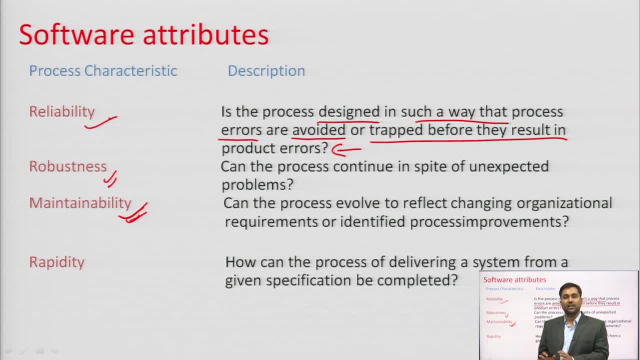 if we will test in the module, if we will test the bug, then we will rectify the same module. then all the problem will be solved. if they are dependent on each other, then the chances of reaching in one or the other module will increase. that is why we try. 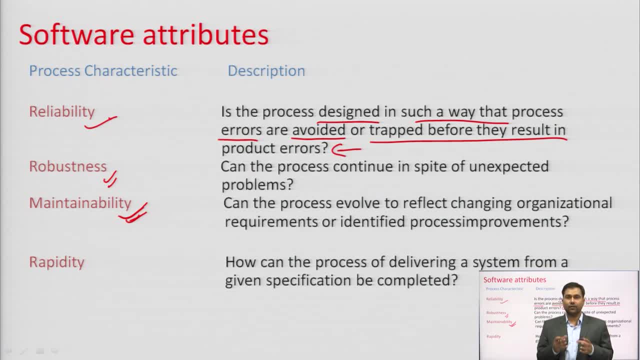 to apply the modular approach. like, for example, if you want to understand in layman language, then there is a bike, there is a bike or cycle, right. then the chain got spoilt in the cycle. then the chain got spoilt in the cycle, the brake got spoilt in the cycle. 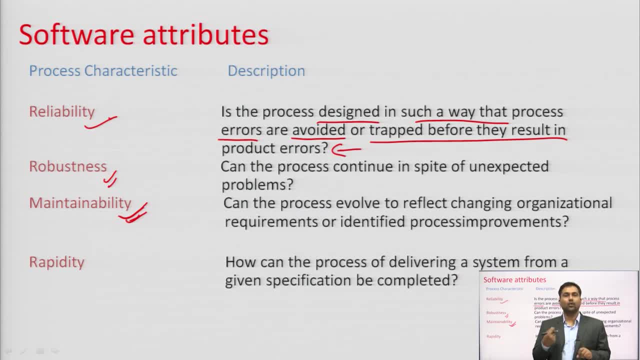 the accelerator got spoilt, the clutch wire got spoilt, then we change the wire. if the piston got spoilt, then we change the piston, not the whole engine. that is the modular approach. everything is combined, assembled and the bike is ready. the tyre got spoilt, the rim got spoilt. 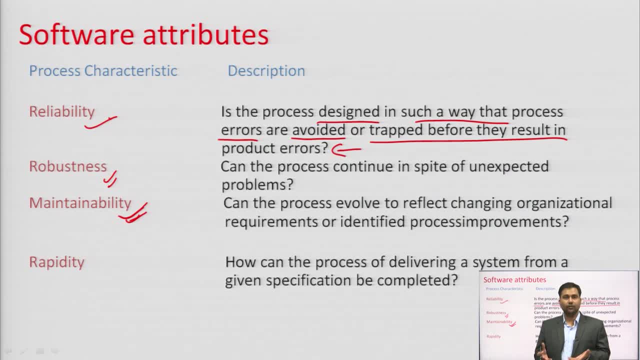 the handle got spoilt, the tank is leaking- anything fuel is leaking, so we will fix that particular problem, not that we will rectify the bike. same process applied in the modular approach in the software development. if we have broken in different modules, then we will focus on the particular module. 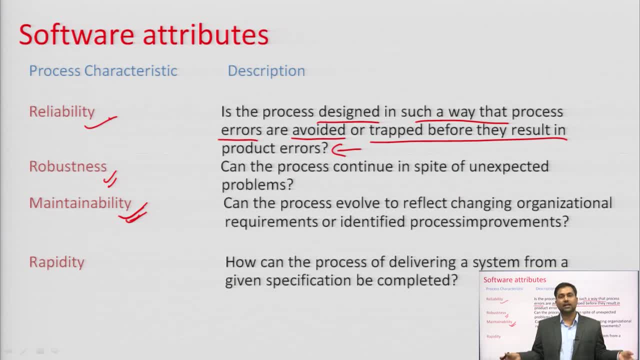 to find out the bugs and remove them, not that we will increase the time cost of all the code. that is why always go for the modular approach and rectify the particular module which has bugs and errors. then the maintainability will be easy. if there are any bugs, then we have to change the module. 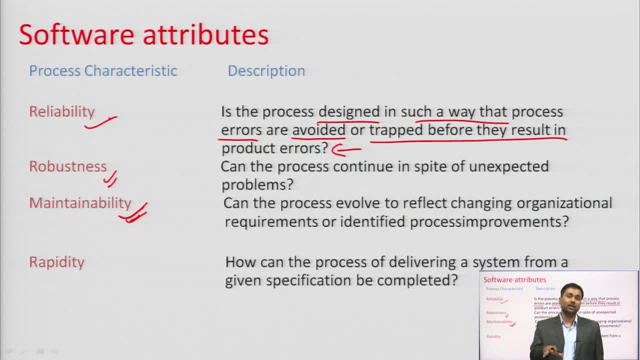 the team has to focus on the person who worked on it. if the person worked on the particular module, then the person who worked on it, the whole team, will be free. they will not have to pay extra salary, so the time, cost and maintainability will be easy. 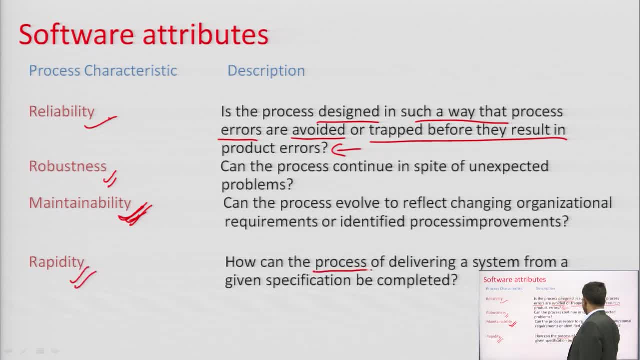 rapid. how can change the process, delivery and system from a given specification to be completed? so whatever rapid development we have in the modular approach, if we are independent, we have a module, then put different team and start the development. when we divided the whole process in the different modules. 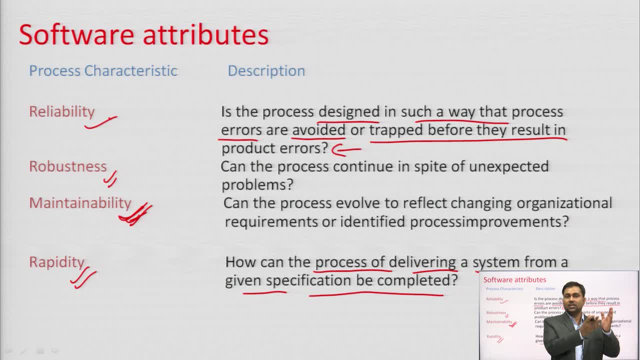 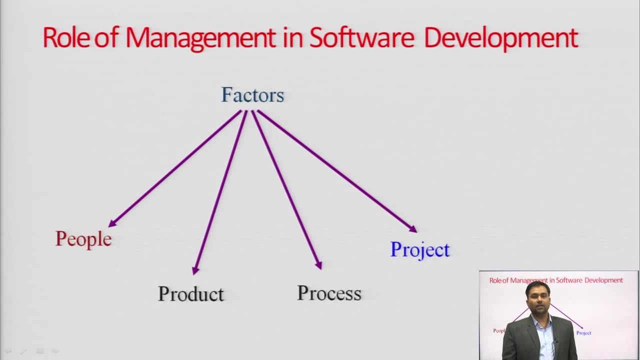 and each and every module assigned to the team and that team responsible and accountable for that module only, and after that integrate all the modules in the timeline manner and delivered the project right. this is rapid development. we will teach you future. next RAD model. rapid application development model. 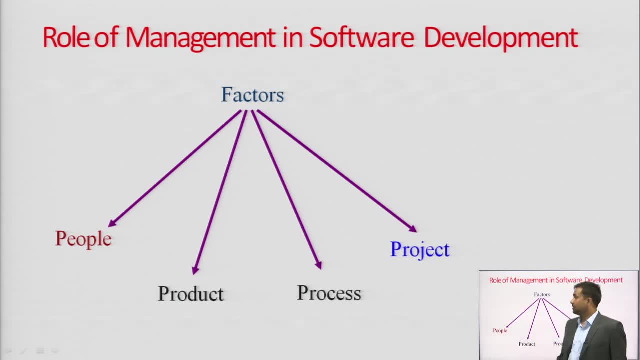 role of management in software development. you are seeing four P's here. four P's: what are they? people, product process and project. these are the four P's factor of the software development process. people means human resource, which is the software technical skill which will be applied. the technical person will help in software development. 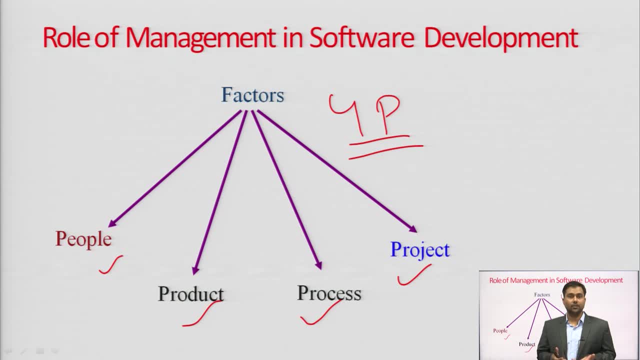 will develop? what will be the product? what are the software quality attributes? what are defined by the client customers? what process we are applying to develop? we are applying waterfall model? we are applying spiral model? we are applying automation testing or we are applying agile process, or we are applying manual testing? 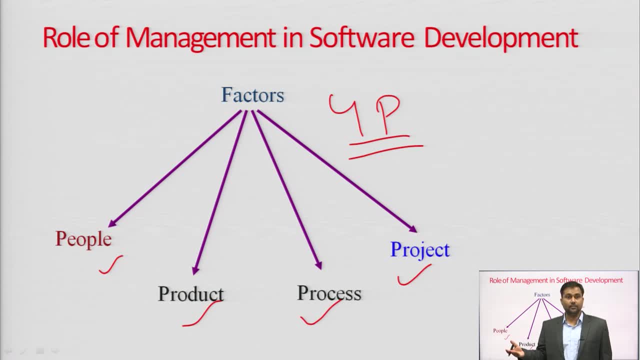 right. what are the quality checking parameters at the release time? what is the life cycle of the whole project? what is the delivery at the time? modules to be delivered or complete project to be delivered depends on the process to process each and every thing. four P's are dependent on the quality. 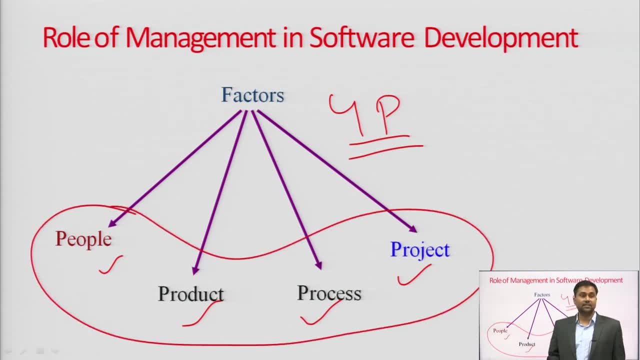 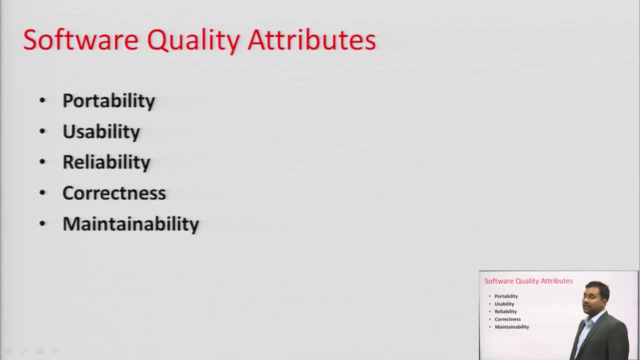 all, all four P's. what do they decide the quality of any project? this role is very important for the resources in the software project. software quality attributes: portability, usability, reliability, correctness, maintainability, maintainability and reliability. I have already told you how usable is the software right? 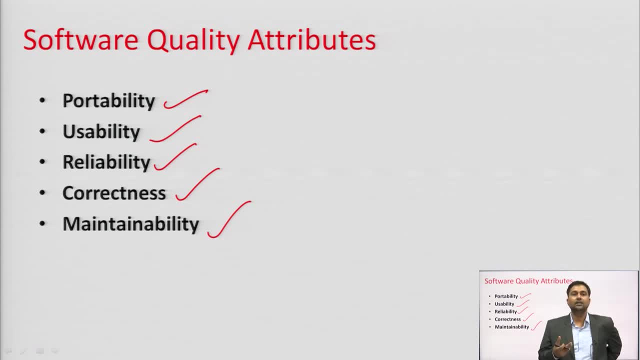 all the social networking websites. you are seeing whatsapp. you are seeing these educated and maximum people are using even. you see the payment gateways through UPI means you don't have to write anything, you don't have to enter anything, simply you scan and your payment is done. 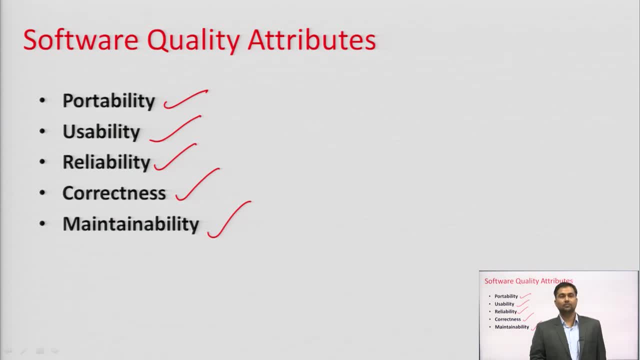 if you have money in your wallet, that is what. how good is this? UI right, usability. everyone is able to use that software, that mobile application, easily. every person is taking transition on their mobile and doing shopping. go to any shop, go to paytm, google pay, phone pay, etc. 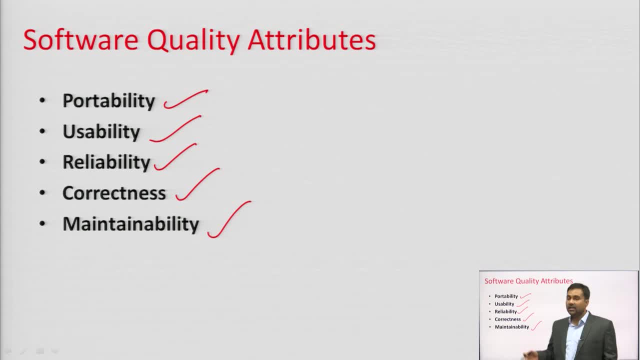 all are payment gateways. portability, portability- portability means to run one software code on different operating system or you can install software pendrive anywhere. you can download and install anywhere. it is portable. right portability. but normal civil engineering. you can't take bridge anywhere. 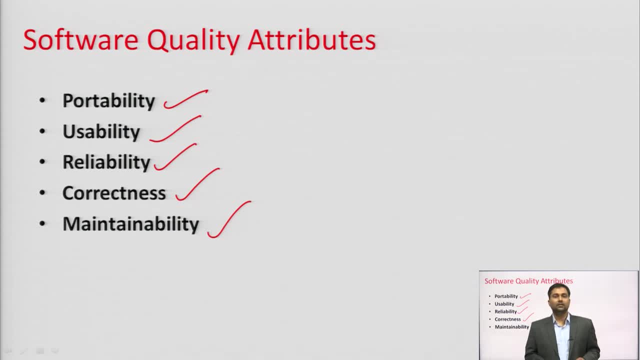 you can't take bike anywhere, right, all are the engineering product. but in software field, software is portable. you can install anywhere if its system is compatible. compatibility is a must, right, if we are doing any programming on java platform, then platform is independent. it will run on every operating system. 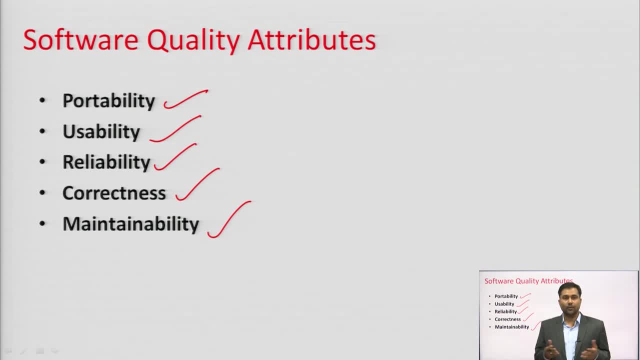 there should be byte codes, simple. there should be executable byte codes. if it is proper in systematic way, whatever was our problem- it has been provided as a software solution- then it will run on each and every software current existing operating system. it will run on everything that is portability also. 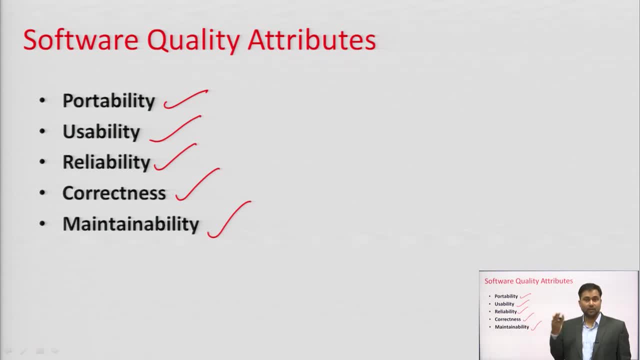 right, achieve portability. how much it is it will depend on programming language, but our software is portable, right, and I have told you about reliability, correctness. if there is any bug, if there is any defect, if there is any problem, we feel that client is not satisfied or our testing team is saying: 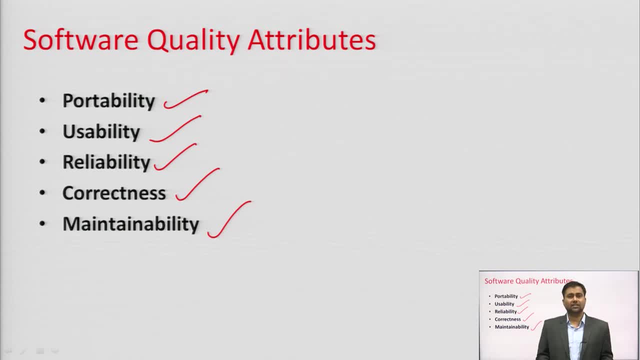 that there should be changes and we feel that we can easily correct. there should be correctness. by that correctness we don't have to change the entire software, we don't have to change the entire module, simple line of codes. or if we change the program then the entire project should be correct. 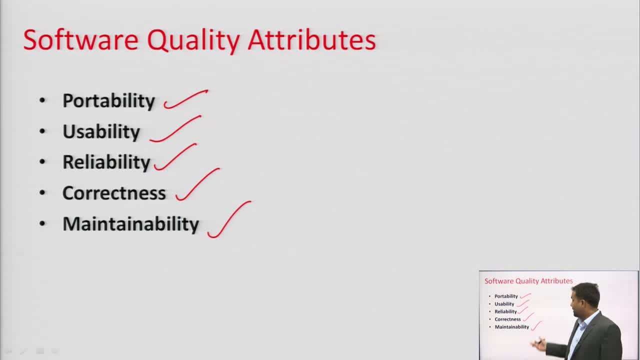 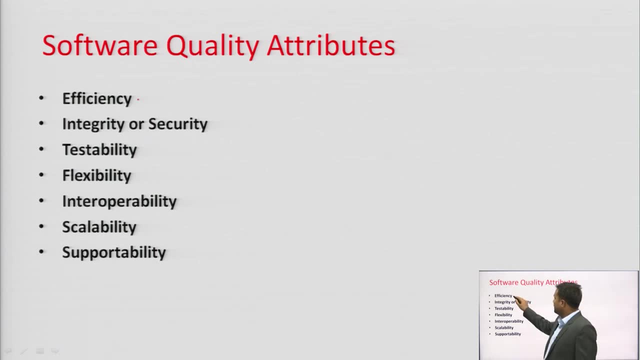 right, that is the beauty of modularity. also right, I have told you about maintainability and few more quality attributes, right. so in the software efficiency, when we check the efficiency by doing response time, by doing multiple performance testing, by doing compatibility testing, by doing configuration testing, right, 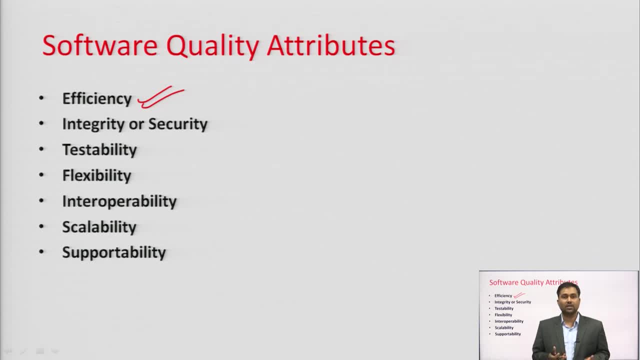 any bugs are not coming. any software is not crashing. any program is not crashing. all the proper response is coming. time, complexity, space complexity is reduced or not. any bugs are not coming due to integration. any compatibility issue is not coming. response time is not decreasing. right time come toni hora load honi me ja time, toni lag raha hai software, each and everything. 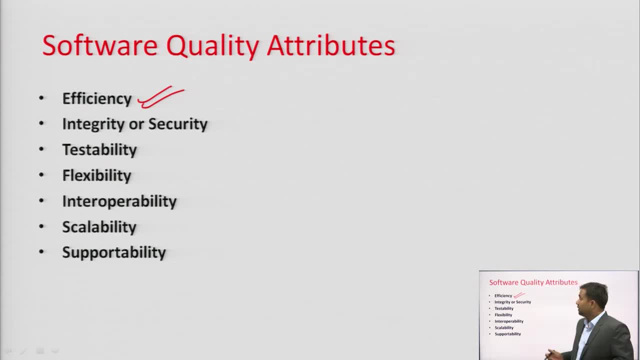 is the parameter of efficiency of the software, integrity of or security. that is the most important concern in the software field: cyber security. bahus logon naam suna hoga, but security provide karna different, different softwares machine, internet banking ka software, payment gateways hai multiple log apne wallet, bank sub ke phone me hai, basically saare transaction. 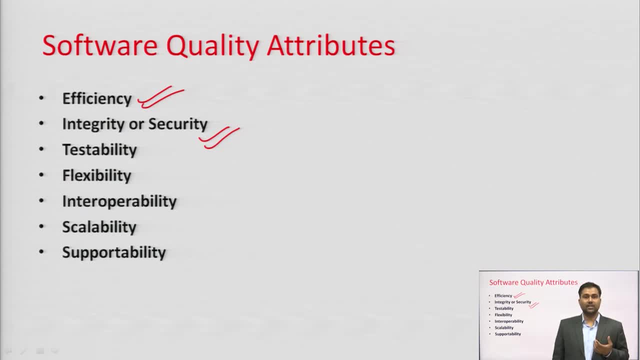 online hi chal rahe hai to security. major concern hai right to security, major concern hai to security, integrity, accountability. mohot important hai humare liye right testability, agar humne modular approach main thotir pehle explain kara, agar humne modular approach apply. 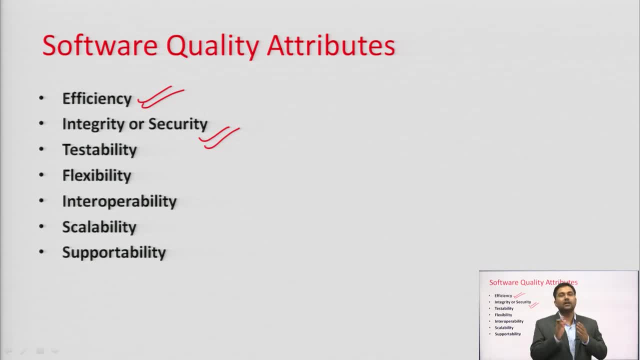 kar rakh hi hai to ek module me error aayegi. dusre me nahi aayegi, testability asan ho gai. isko check kar liya, yaha pe bugs hai. is wale module me bugs hai. agar suppose that module number m1, m2 and m3 apas me ye connected to hain but a lot of the software. 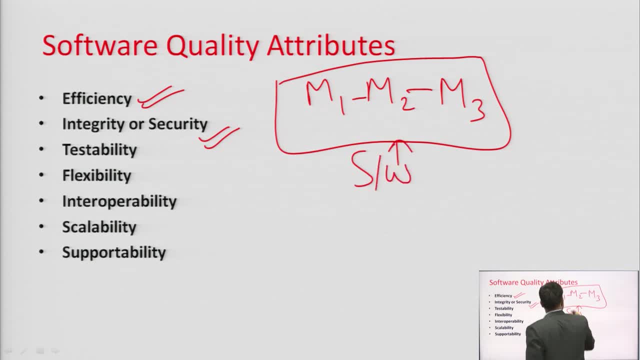 modules right, but m1 me, m2 me koi bug aayi, ya error aayi or bug, then m1 or m2 me, wo bug nahi aayegi, aane ki chances kam hai, agar ye maalo, ye chatting module hota facebook ka. 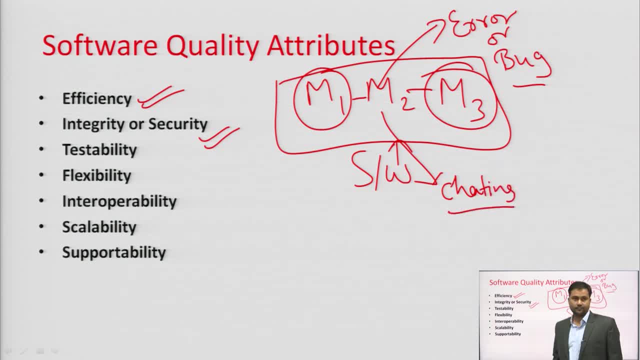 ok, ok. ok, so testability, sihr hume bug aayi hai, chat message maalo nahi ja rahe hai to hum chatting ke program check karenge na ki photo ke profile ke ya login page ke testability aasan ho jayegi. 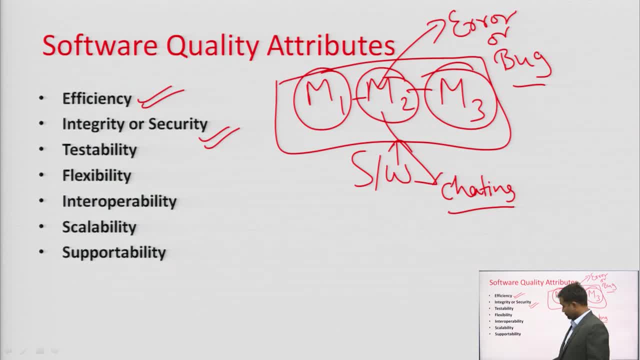 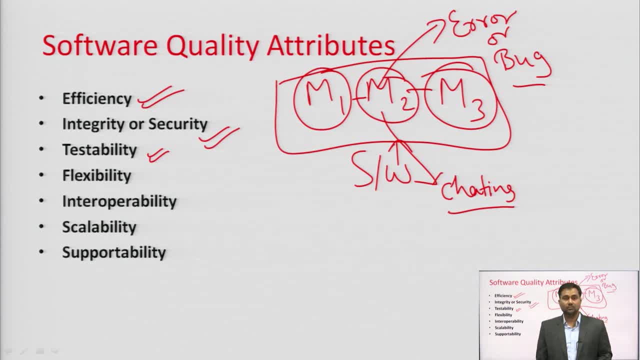 So if printf is not able to print something, then printf is defined in conioh or scanf is defined. So developers need to check that, not that they check graphh or mathh. that is the modularity of software and programs. 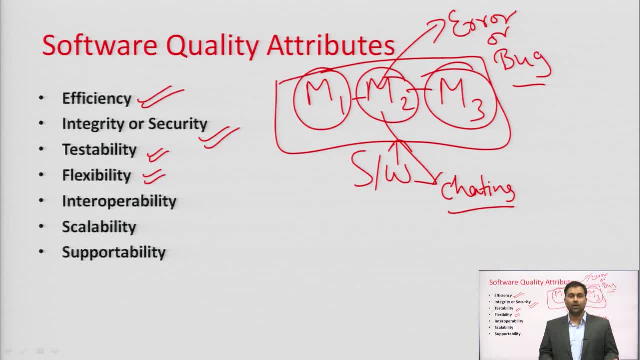 Flexibility. obviously I told you that code is flexible. change any code, add, update or remove, then functionality will be removed or added, depends on your problem. to problem: Interoperability: multiple different procedures are connected to each other, if you have seen. 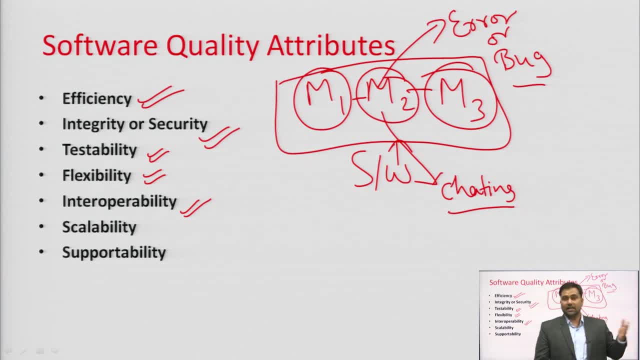 online website. then what is there in online website? client-serve architecture is there, but along with that, accountability responsibility is increasing on login page, of whose security that only authentic person can login. That is proper. It is provided by the password right. it is validated on the database on the backend. 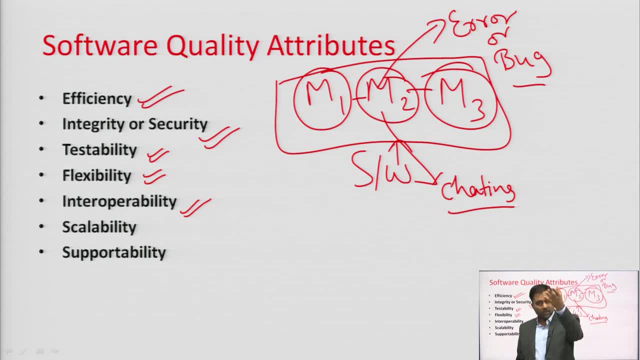 Again, when you do the shopping after adding in the court, the methodology of the bill should be proper. there should not be more or less in the bill. if it is less, then the company has loss. if it is more, then the customer has loss in both the cases. 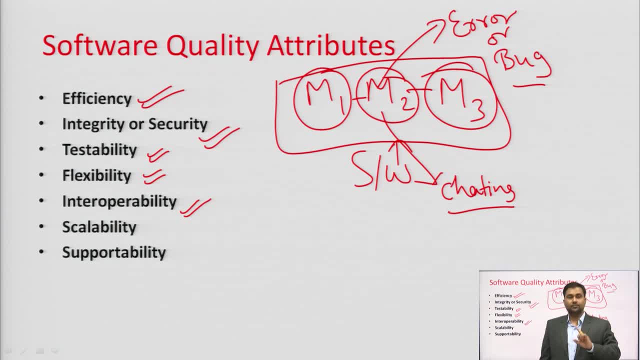 the company has loss because the customer will lose After that. payment gateway third party- right. sometimes there is paypal. there is multiple rupees, multiple third party which secures the payment In row, but the payment is secure, provided to some the online transactions, UPI at. 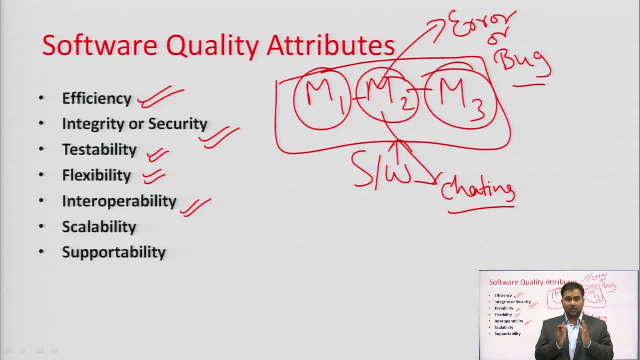 Google Pay, Paytm, phone pay by the third party is it is on Amazon, on Flipkart, none of the Hazlip. everyone has payment gateway but their third party. but they are connected to each other. they all have connected at that time. it is all of the parts of the software. 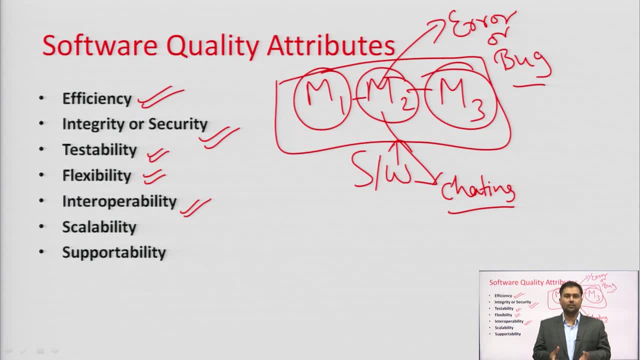 component? what software, However? website of online shopping. if payment gateway is attached, it means that means all of the parts of the payment gateway. Everything is connected. Now this is providing you payment gateway, The online, The th hope, Then thisag概. and paypal transaction is also knee under. 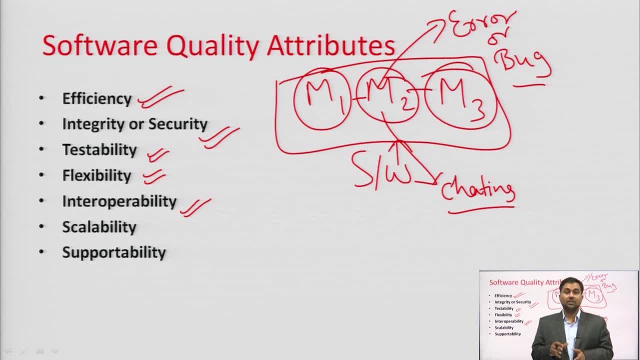 that software component and they are completing a project together. then only online shopping can be done. and scalability. have you ever seen that? how many new accounts can be created on facebook, any idea? all over the world the load on the server is increasing. if you see a college investment. 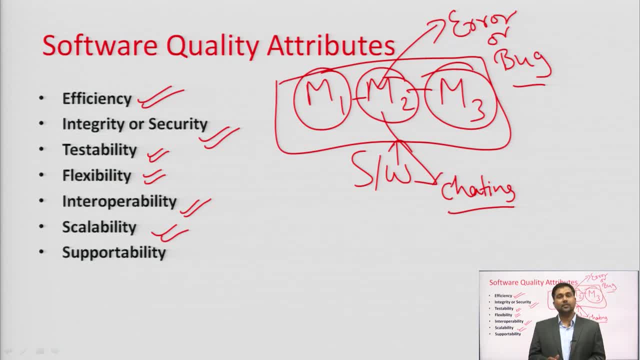 you will know how many seats are available, how many students will come in the next year. here scalability software can be done, but the social networking websites like amazon. you must have seen that once on flipkart pen drive was sold in 1 rupee. there was an offer. 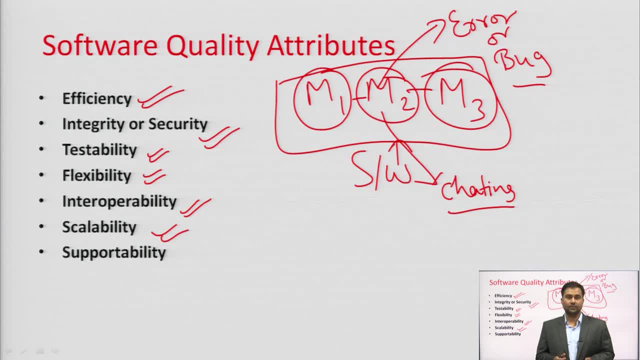 then flipkart's software crashed. so what happened? scalability was not proper. the server had to be extended. if we have so much load at once, then the software should not crash. our website should not crash, so scalability should be there. expandable means as the number of users increases. 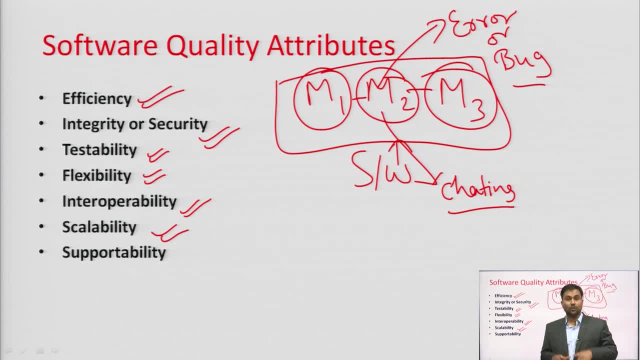 the load balancing will be proper. number of servers should be there which can handle the load on the backend. so this is also a challenge. scalability is a tough task. quality is a major parameter. it should be scalable and we have to pre-define how much load can come. 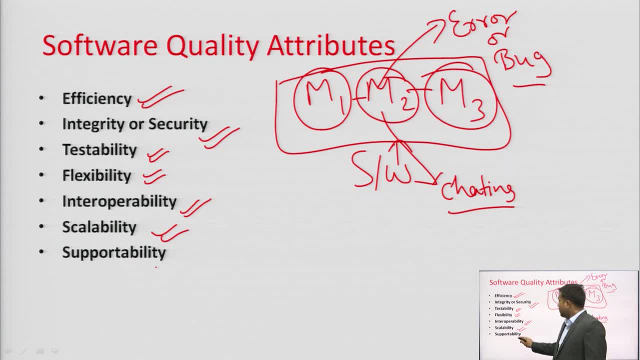 the prediction should be one right: supportability. whatever challenges we face in the run time, there should be support system. in the current time. if our software crashes, then our technical team or anyone who can remove the bug quickly. support system: if there is any problem, then customer care. 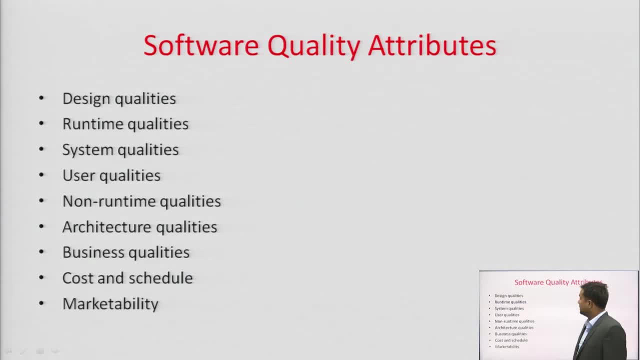 that is why we are made right for support and attributes of software. quality, design qualities- I told you it should be modular approach. run time qualities- if there are no bugs or errors in run time, then you can see system qualities. configuration, hardware configuration, RAM, ROM, cache memory, whatever things are required. 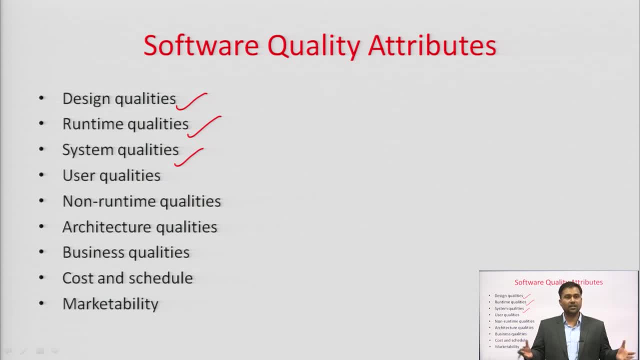 processing speed, operating system, operating system, each and everything, whatever support system is system, that quality should be proper user quality. now it depends that banking, banking software which people are using, user quality should be good. it is not necessary that every software should be made for everyone. some software are made for scientists. 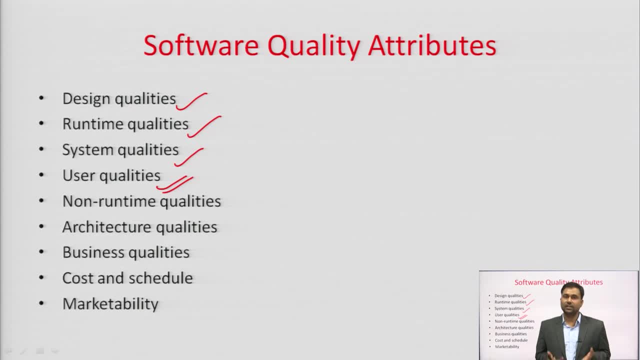 and researchers. all of us cannot do coding. software engineers who develop knowledge of coding, only they can do. that is also software right. so the quality of user should be different for different software should be different. it happens right: run time, non run time, qualities without run time, if any software. 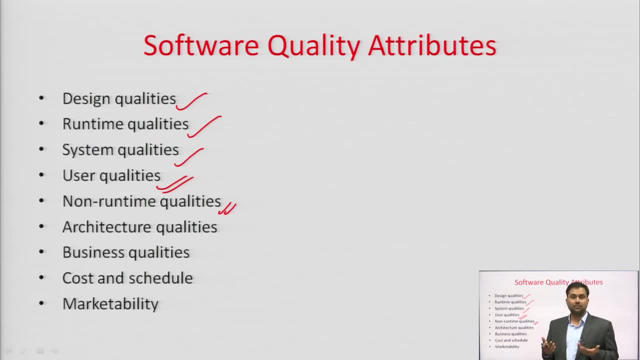 memory is full crashed. right memory is leakage, right vulnerability is coming somewhere. so by checking that, otherwise that also will effect on quality. if your memory is full, software crashed, whereas there was no problem in coding. either memory is less or in multiple time back end garbage memory is occupied. 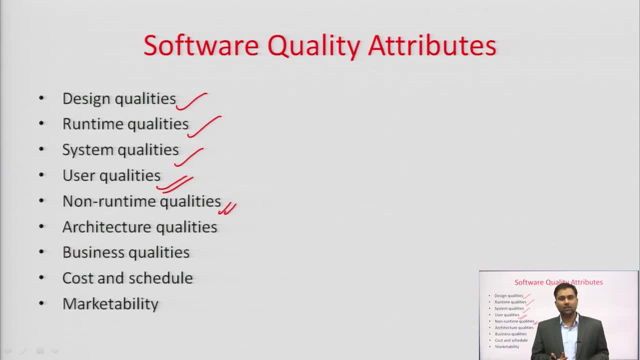 that is called in technical term, technical pointer through dangling pointer. so there, memory is occupied through dangling pointer. many times now that comes when memory is occupied and software is crashed. right, that is also type of error and bug, but in case of java it is garbage collector: free memory. 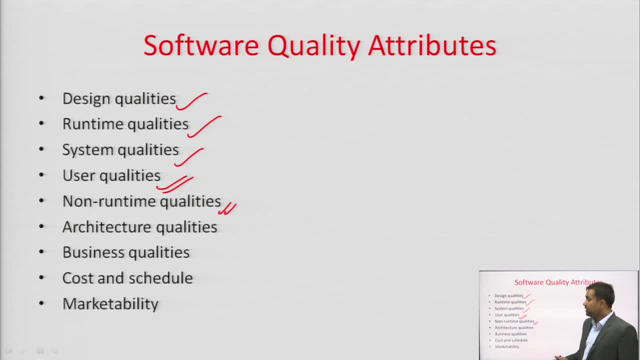 it is free. that is solution in java, right, but leave it. architecture quality software architecture modeler should be. I will tell further. design document design and business quality, business generation, business, business logic. like business point of view. like if on amazon website image is not good but bill should be generated properly. 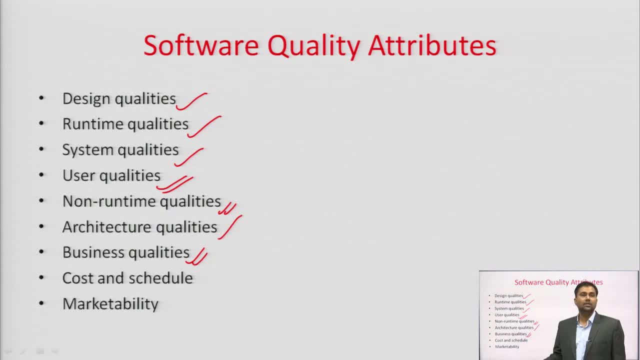 transaction should be proper, profit will not come, people will not be able to do shopping right, business quality proper, multiple time check, multiple testing should be cost and scheduling our fixed budget, which we took budget in that only project should be complete and scheduling, which we did according to that. 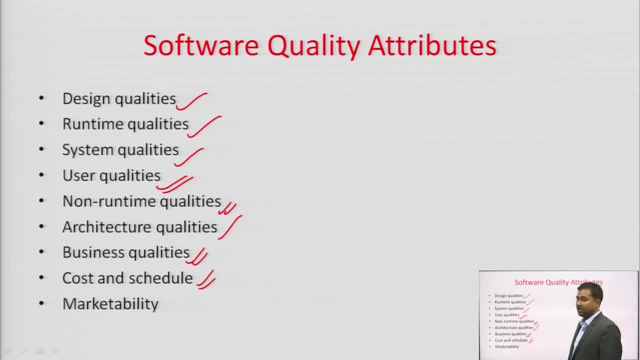 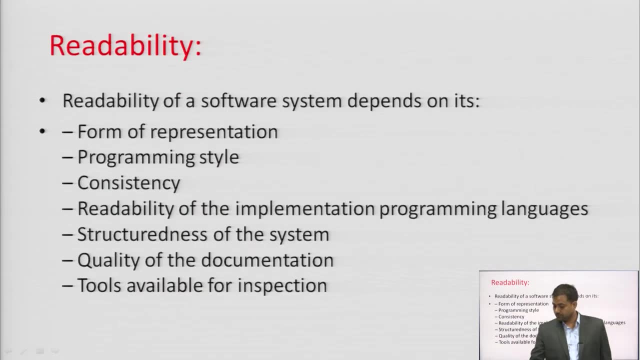 delivery should be done in timely manner. that is also part of quality attributes, and marketability means market should not be outdated. whatever is our market, accordingly, things should be updated right. so basically so readability: whatever things we have written on software should be proper, readable form of the. 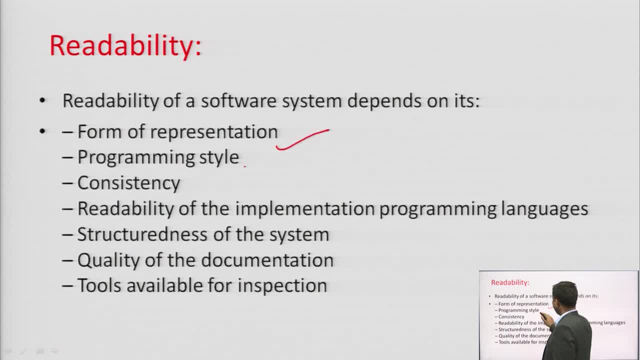 representation, programming style, consistency and consistency. there should be proper consistency in the flow. it should not be written anywhere, isn't it? readability of the implementation programming language. that is why you write comment line that we don't understand the code in which we have coded the naming convention. 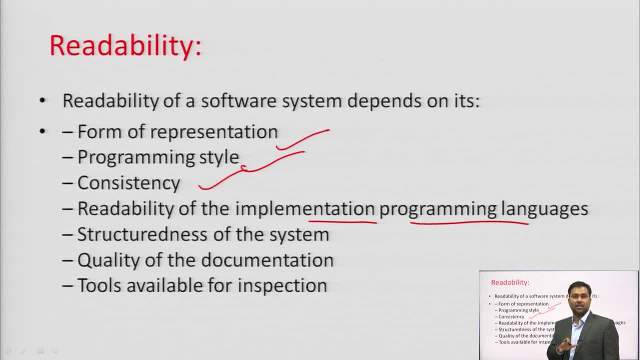 which we follow should match with proper requirements and code. it should not be that you are adding code. you have written a function, some other- ram rahim- so it will not be understood why you have made this function. but you have written add. it will be understood. 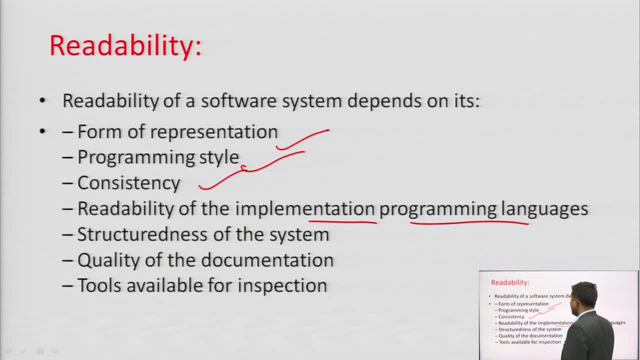 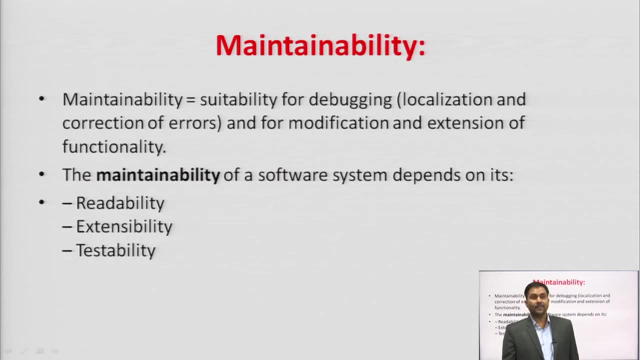 that this function is made to add numbers right. structure of the system. quality of the all the document should be quality wise. proper standard formats should be documentation and tool. availability of inspection: any tool availability should have proper inspection right. maintainability: I have told you again maintainability. 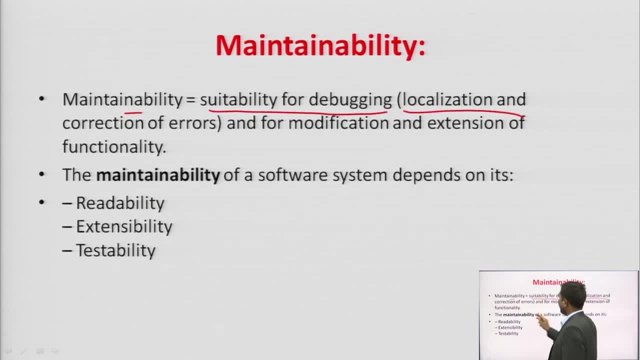 is equal to suitable of debugging, localization and correction of errors. I have told you what is maintainability: find out the bug, any particular localization means in any particular localization. when the bug will fail, when the modeler approach will apply and try to keep the modeler maximum independent. 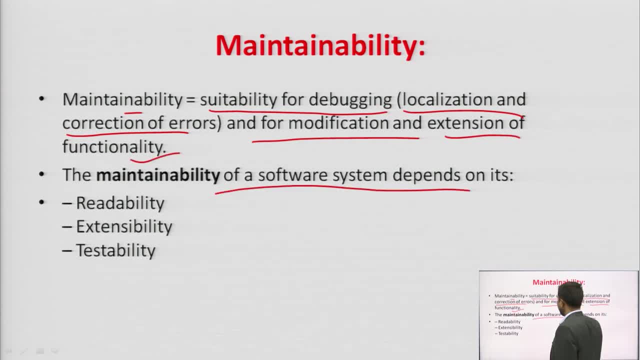 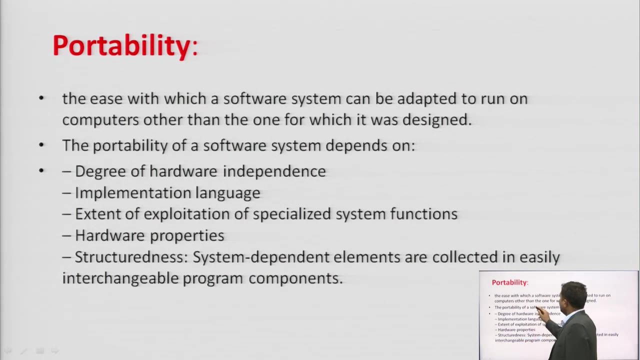 right and modification and extension of the functionality. maintainability of the software and dependent on the readability, extendability and testability. these three factors will depend on maintainability, readability, extensibility and testability. if testability is good, maintainability is good right portability on computers rather than the one which is designed. 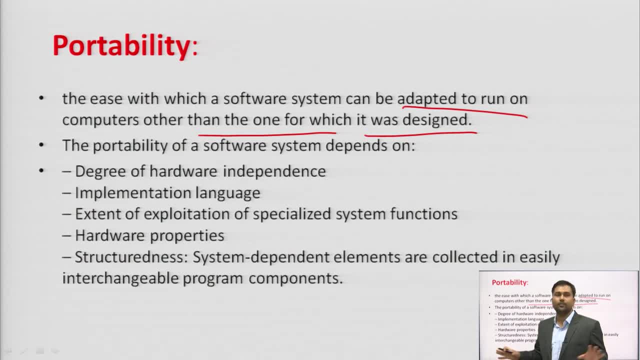 for which it is designed. it should run on other also. it is not like that it is running on one operating system. rest of the operating system user will not be able to use your software, so it should be portable. it should run on every system and portability of the software.